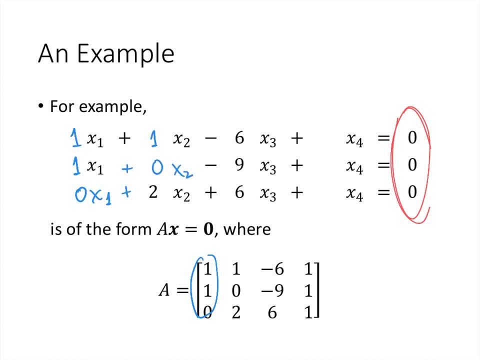 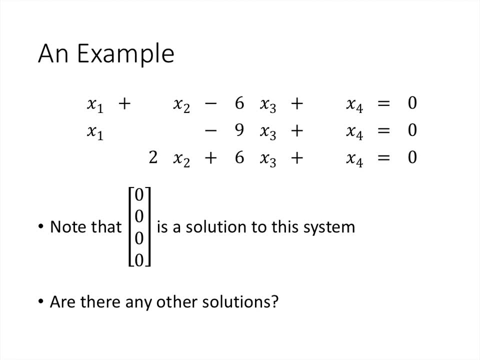 For X2, we have 1X2,, 0X2, and 2X2, and that's why our second column is 1,, 0,, 2, and so on. Now, if we look carefully at this system of linear equations- because all of the right-hand side numbers are 0s- 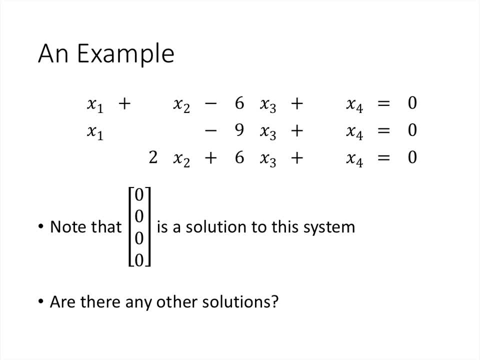 one nice feature of homogeneous systems is that the 0 vector is always going to be a solution. If we plug in 0 for all of the variables, then of course we will get 0 on the right-hand side, And so that's just a feature of homogeneous linear systems is that the 0 vector is always going to be a solution. 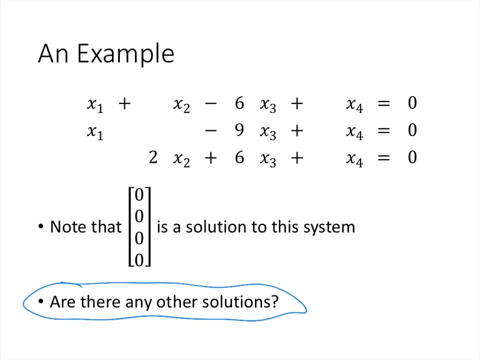 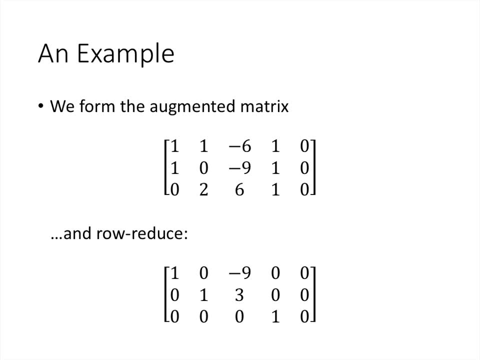 So here's the real question, though: Are there any other solutions, And if so, what are they? Well, the way we're going to answer that question is the way that we've been doing all along. We're going to form the augmented matrix and row reduce. 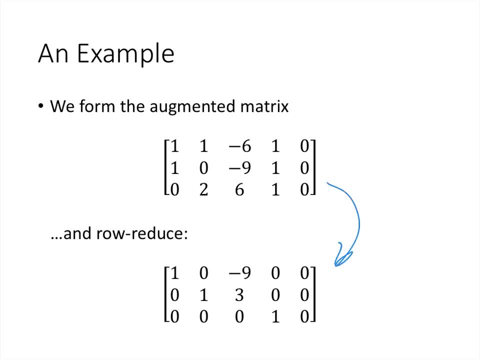 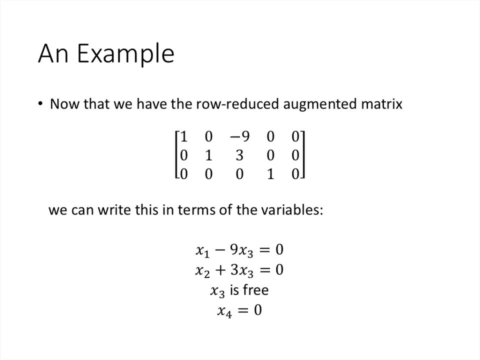 So again, I'm saving you the trouble here, but this is going to be the row reduction process that we've been talking about, And here's our reduced row echelon form And we can take that. We can take the row reduced augmented matrix and write it in terms of the variables. 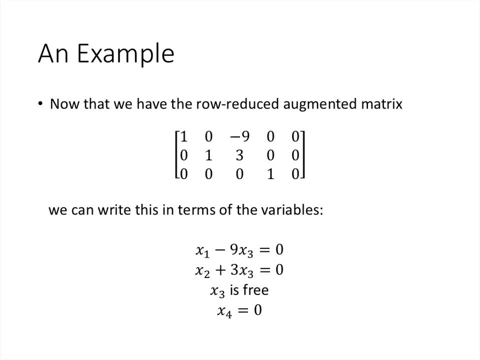 So all we're doing there is taking each row of that matrix and writing it as an equation. So in the first row I have 1x1,, 0x2s, negative 9x3s and 0x4s. 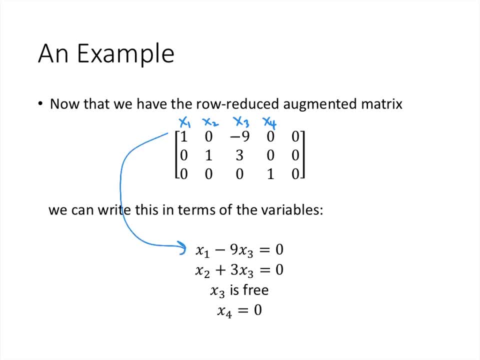 And so I just write that in the equation form as: x1 minus 9x3 equals 0. Now x3 here is a free variable, because there's no pivot in that x3 column, And so we write that simply using the words: x3 is free. 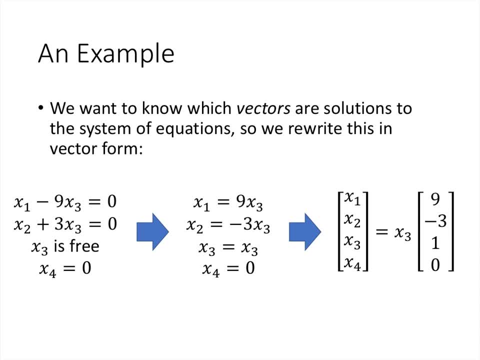 Now we're going to do something a little bit different than we've done in the past, Because what we want to know are which vectors are solutions to the system of linear equations? We want to write our solution in vector form, So here are the equations that we have from the previous step. 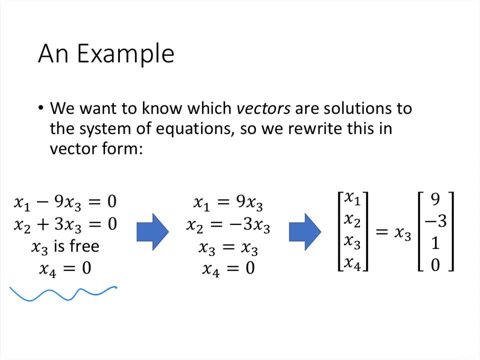 And what we want to do is solve each of those equations for the basic variables. So x1,, x2, and x4 are our basic variables. Those are the variables corresponding to the columns where we had pivots, And so x1 minus 9x3 equals 0. 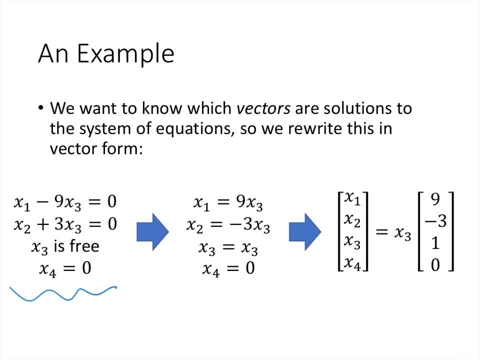 I'm going to solve that for x1 and write it as x1 equals 9x3.. Similarly, I'll write: x2 equals negative 3x3.. Now what do I do with a free variable? Well, let's just write that as x3 equals x3.. 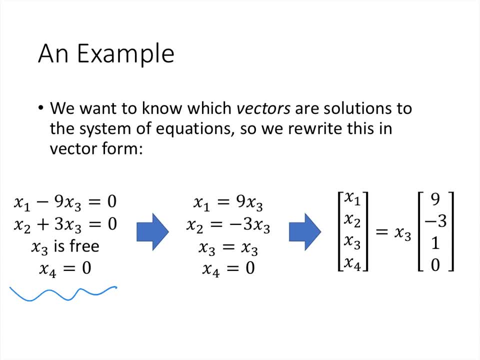 It's not really saying much, but it's just going to help us in the next step. And then x4 equals 0.. So now what I want to write this is a vector equation. So I've got x1 through x4 here. 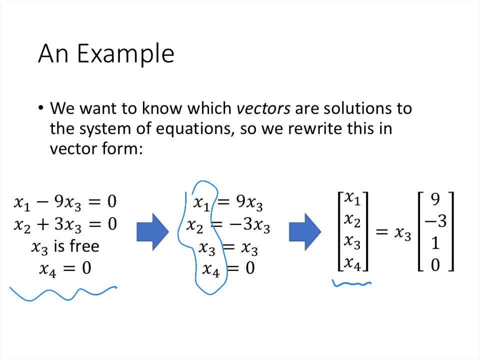 And so I'm just going to put those together into a vector. And now what I will also want to do is write the solution as a vector, So 9x3, negative, 3x3,, x3, and 0. I can think of as x3 times the vector 9, negative, 3, 1, 0. 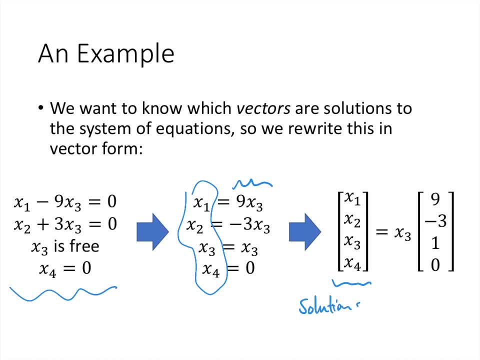 And so, in other words, the solution set is simply all multiples of that single variable, which is, as we've seen, a span, And so we can write the solution set as the span of that vector, The span of 9, negative 3, 1, 0. 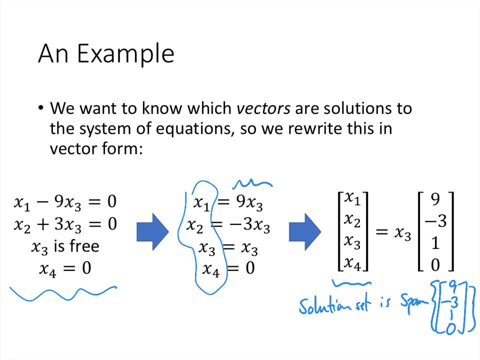 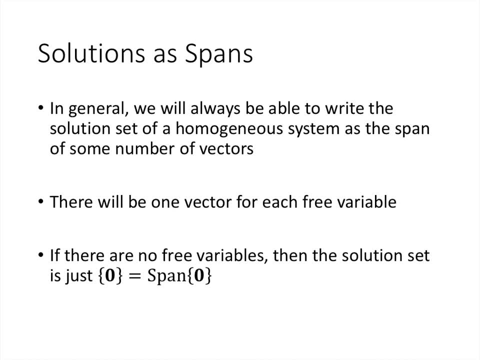 If we had had more free variables we would have more vectors to write down for our span. So in general, we're always going to be able to write the solution set of a homogeneous system as the span of some number of vectors. There's going to be one vector for each free variable. 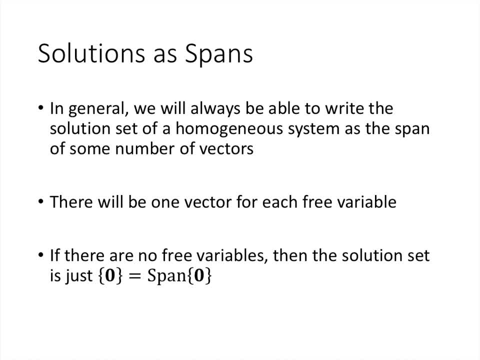 And if there happened to be no free variables, then that zero vector, the thing that's always going to be a solution, In fact that will turn out to be the only solution. And so the zero vector all by itself, only that one vector, which can be thought of as 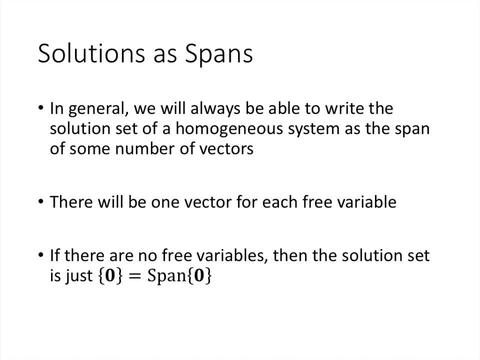 the span of just the zero vector. Remember, as we've seen, the span of a single vector is just all multiples of that vector. But if you multiply the zero vector by any scalar, you just get the zero vector. So span of the zero vector, that's all multiples of the zero vector. 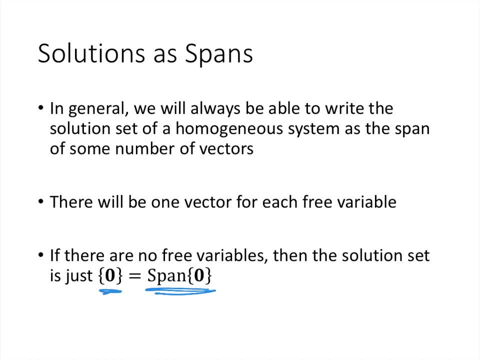 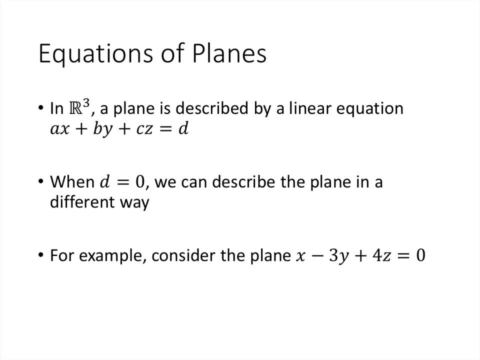 But all of those multiples are really boring. They just give you back the zero vector. One nice application of this is that it gives us a different way to describe equations of planes in three dimensions. So, as you may know, in R3, a plane can be described by a linear equation. 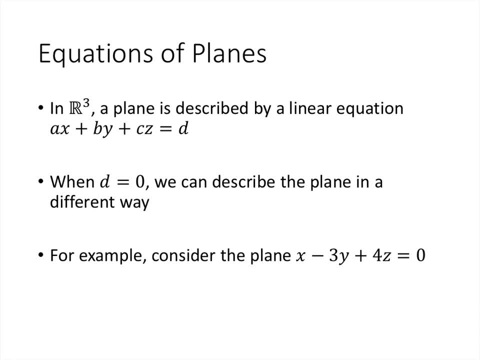 which we can put into the form ax plus by. plus cz equals d, And when d equals zero, that just means that the plane goes through the origin and we can describe the plane in a different way, rather than with that one single equation, which can be useful for certain things. 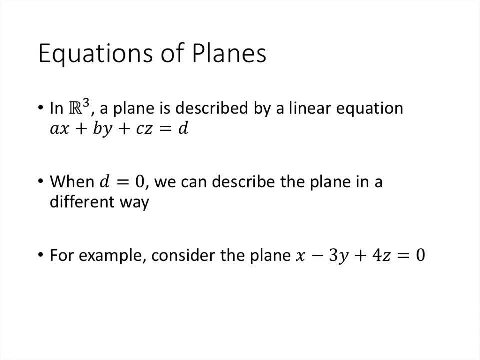 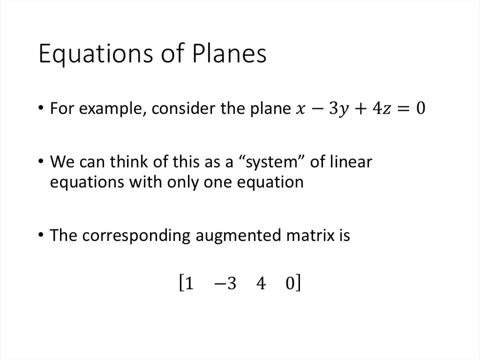 We're going to find a different way to describe it. So, just as an example, let's look at the plane: x minus three, y plus four, z equals zero. We're going to think of that single equation as actually being a system- quote, unquote- system- of linear equations with only one equation. 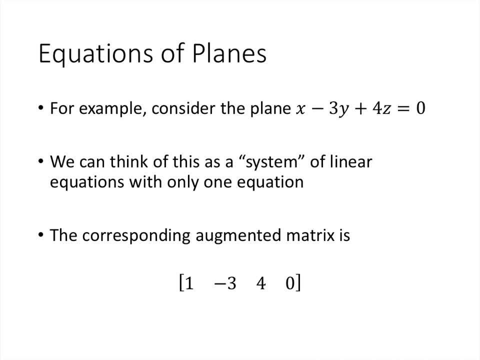 And so we're going to solve that in the normal way, although it's going to seem a little weird, because we only have the one equation, But the corresponding augmented matrix has one row because we only have one equation. one negative, three, four zero. 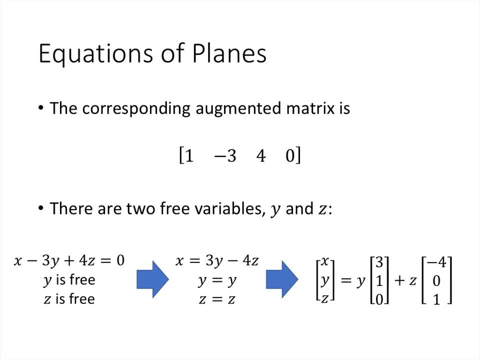 That's already in reduced echelon form, so we don't have any row reduction to do, And so let's just go ahead and write our solution in the form of the variables. So our one row corresponds to the equation x minus three, y plus four, z equals zero. 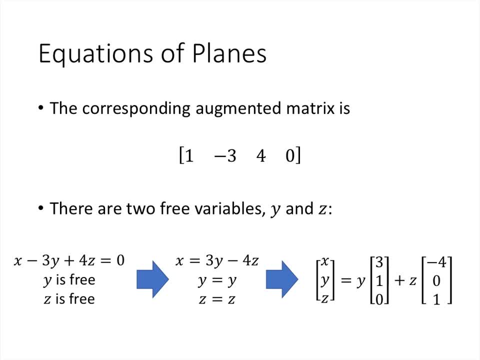 And y and z are both free variables. Following the same process that we did before, we're going to solve our equation for the basic variable. So we get x equals three, y minus four, z y equals y, z equals zero. So when you write this in vector form, 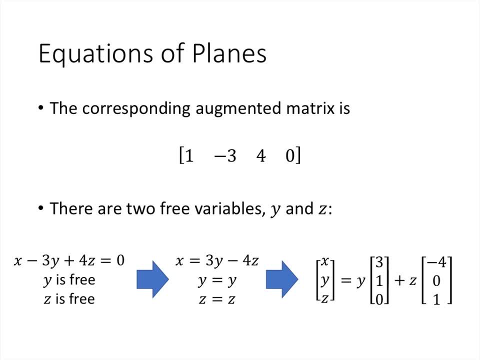 this is actually going to be the span of two vectors. When we write x equals three y minus four z, we're going to break that up into three y and negative four z. Y equals y means we put a one in the second spot of the y vector, but we put a zero in the second spot. 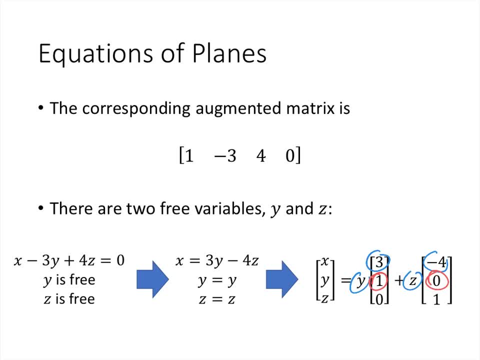 of the z vector, because we don't want to get any z's in that second spot. Z equals z means we put a zero in the y, the third spot for the y vector, because we don't want to get any y's in that third spot. 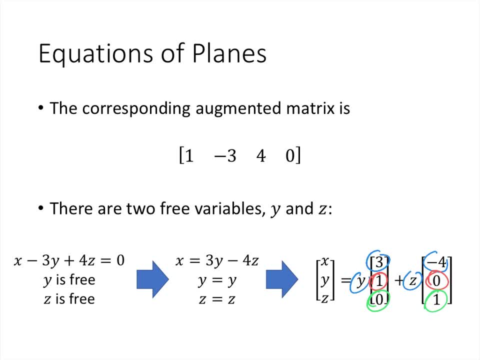 And we put a one in the third spot for the z vector, because we do want to get a z in that third spot. So those are the two vectors that we get: three, one zero and negative, four, zero one. So that allows us to describe this plane in what we call parametric vector form. 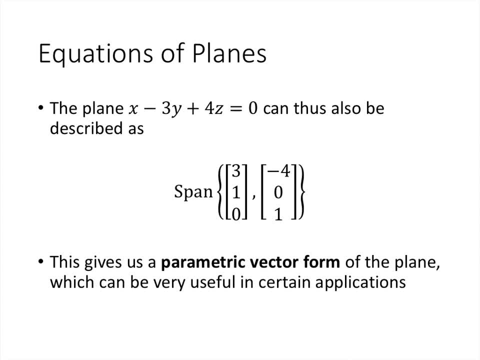 So, rather than just having this equation that tells us x minus three, y plus four, z equals zero. but it doesn't really. that equation doesn't directly give us any of the points on the plane, this parametric vector form does give us a way to generate lots of points on this plane.